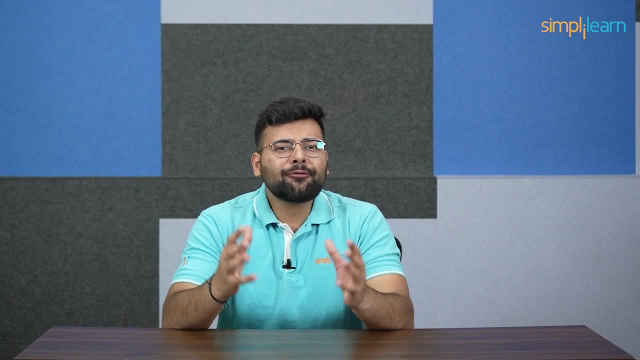 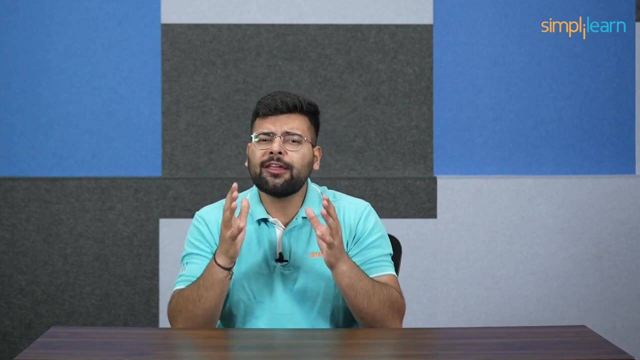 unique purpose and is used to answer a specific question. It is therefore important for data scientists to have a solid understanding of different types of tests and where to use each one in order to draw meaningful conclusions from their data. In summary, statistical testing is an 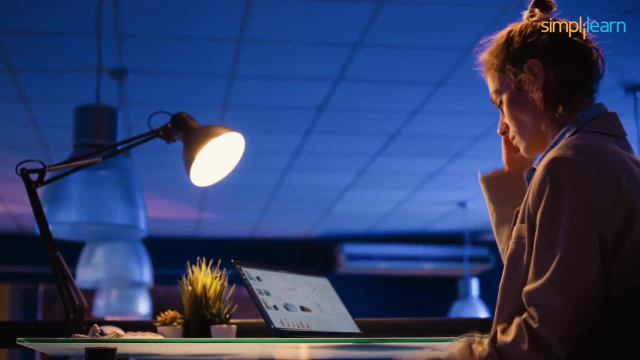 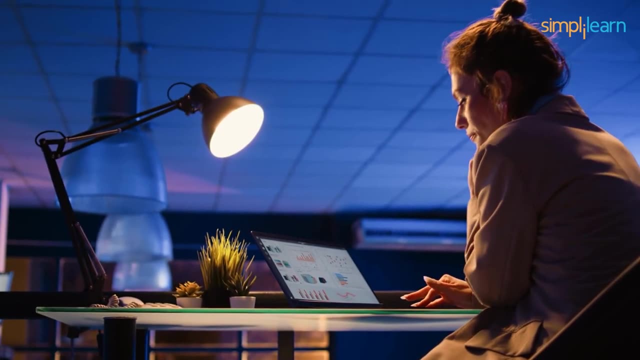 essential tool for data science, providing a systematic and comprehensive approach for exploring and analyzing the data. In the field of data science, statistical testing is a key tool for data science, providing a systematic and comprehensive approach for exploring and analyzing data. It provides insights, confidence and accuracy in the research process, all of which 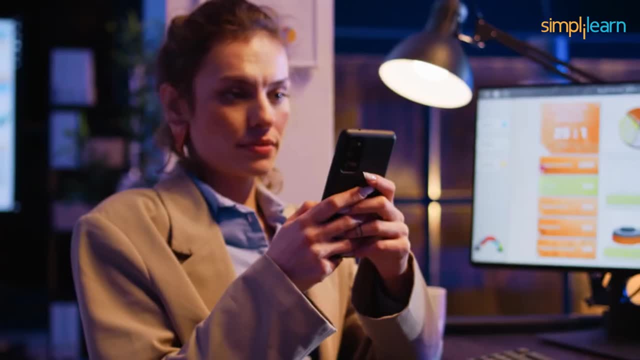 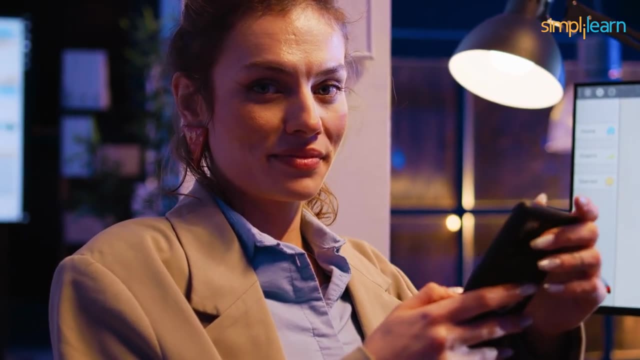 are crucial for making informed decisions based on data. However, it also requires a deep understanding of the test and how to apply them correctly, making it a challenging but rewarding aspect of data science. Hey everyone. so today we will get started by types of statistical testing. 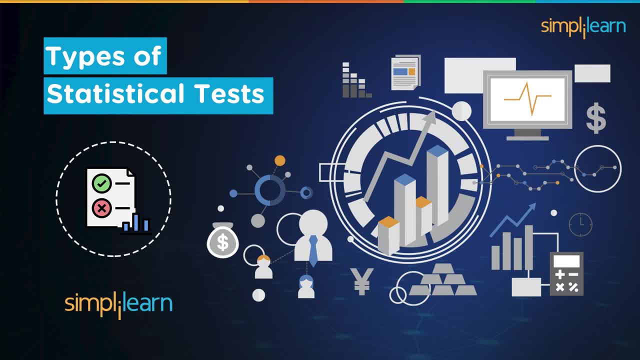 Statistical tests are crucial tools for drawing meaningful conclusions from data. They allow us to uncover patterns, compare groups, assess associations and make informed decisions. From t-tests for comparing means to c-square tests for categorical data, and from correlational tests to regression analysis, statistical tests provide a systematic 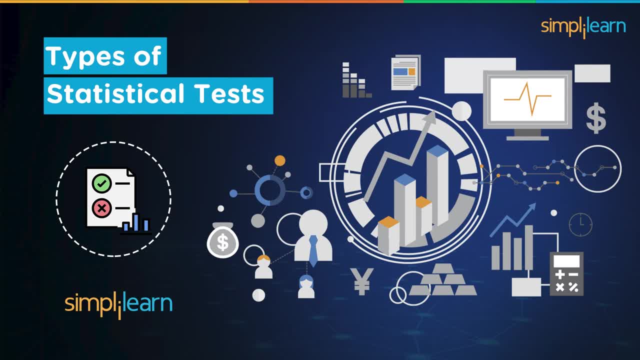 framework for analyzing diverse data types. These tests enable us to explore relationships, identify significant differences, validate hypotheses and uncover hidden insights. By employing the appropriate statistical tests, researchers and analysts can unlock the power of data, unravel complex relationships and conquer complex relationships By employing the appropriate 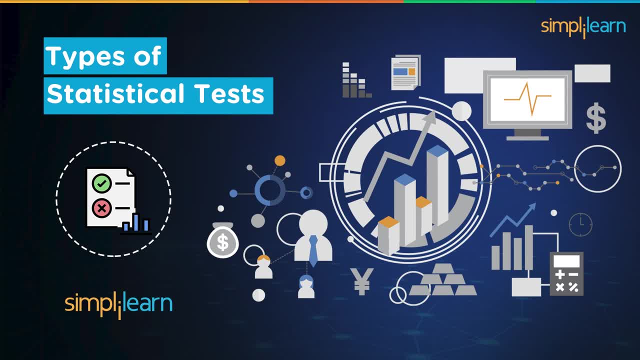 statistical tests, researchers and analysts can unlock the power of data and can confidently make data-driven decisions. Various types of statistical tests are used to analyze and interpret data in order to make statistical inferences. Here are some types of statistical tests, But before we begin, if these are the type of videos that you would like to watch, 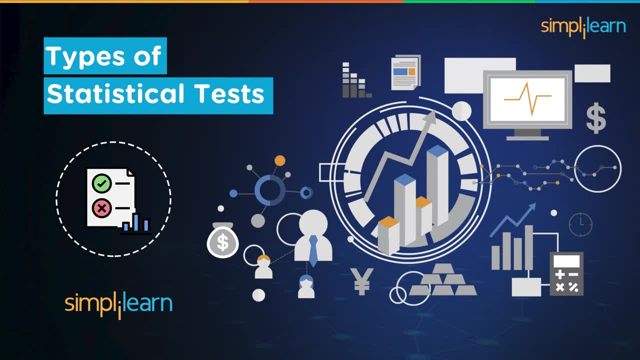 then hit the subscribe button and the bell to get notified on our future content. Also, don't forget to like our videos. And if you are one of the aspiring data scientists looking for online training and certification program from the best universities or a professional 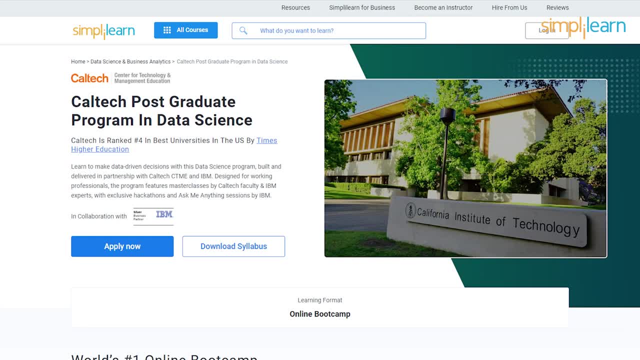 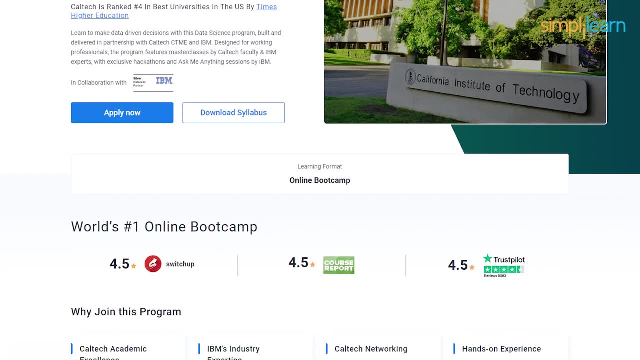 data scientist. looking to switch careers with data science by learning from the best experts, then try giving a shot to SimpliLaw's postgraduate program in data science in collaboration with Caltech University. The link to the program is in the description box below and it should. 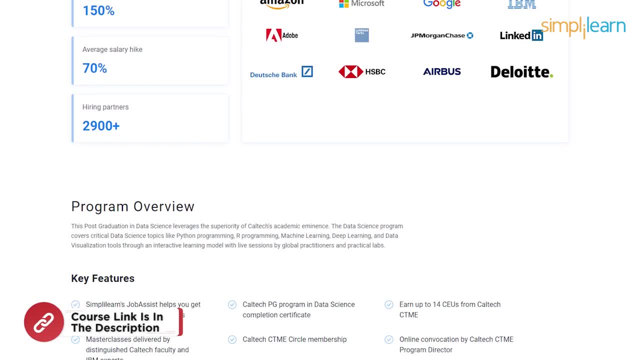 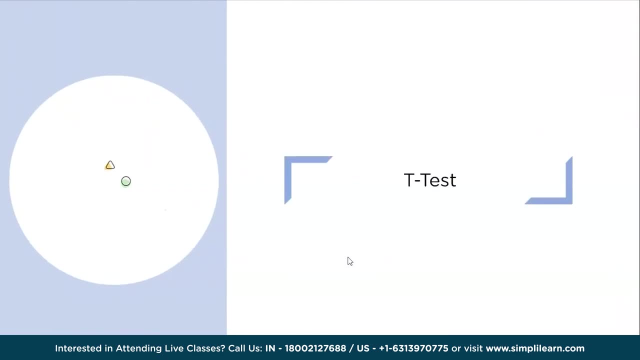 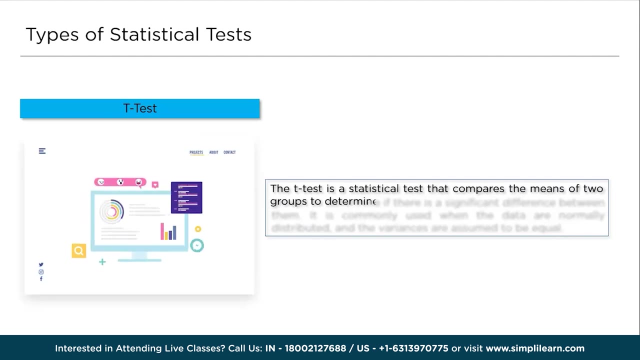 navigate you to the homepage where you can find complete overview of the program being offered. Now back to our statistical tests. So let's begin with the first one, that is, the t-test. The t-test is a statistical test that compares the means of two groups to determine if the 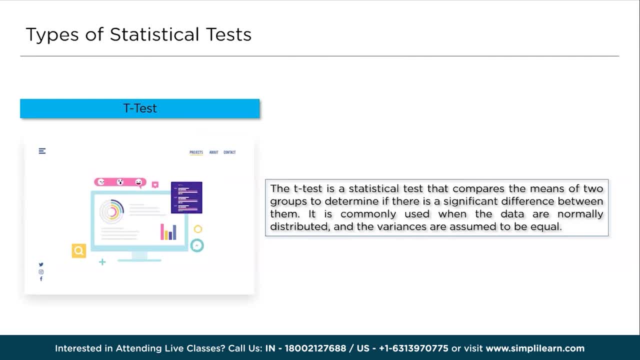 groups are similar or not. The t-test is used when the data is normally distributed. The t-test considers the sample sizes, means and variances of the groups being compared. It produces a t-value and a corresponding p-value, where a smaller p-value indicates. 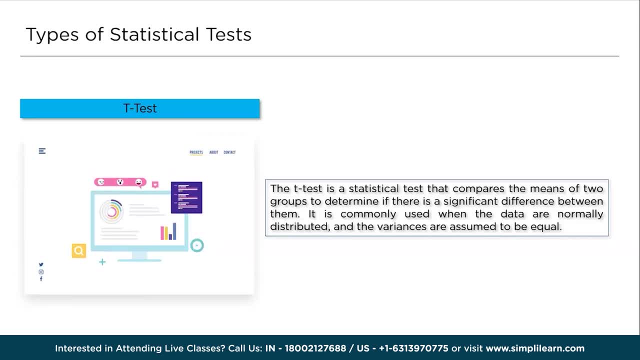 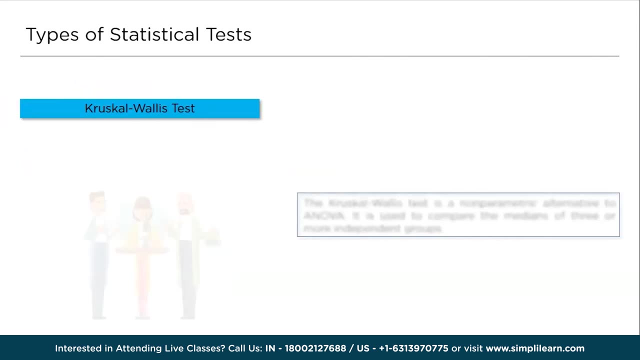 a significant difference, and the t-test is valuable for hypothesis testing and assessing whether the observed difference between groups is likely due to chance or represents a real. Next we have Kruskal-Wallis test. The Kruskal-Wallis test is a non-parametric alternative to ANOVA. 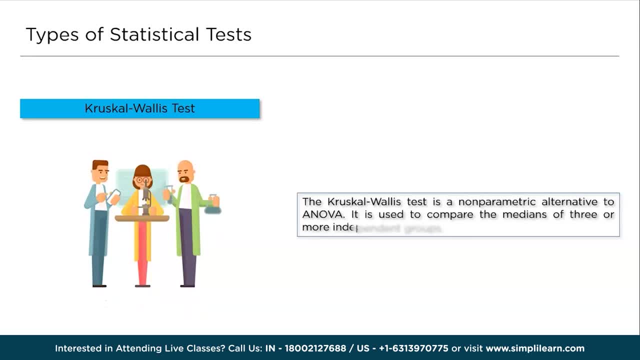 It is used to compare the medians of three or more independent groups. The Kruskal-Wallis test is a non-parametric statistical test used to compare the medians of three or more independent groups. It is an extension of the Mann-Weidner U test for comparing two groups. 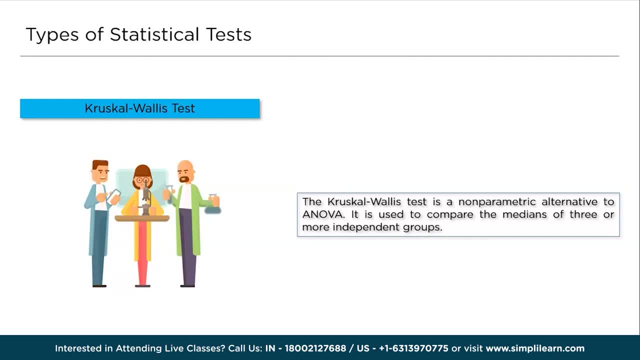 The Kruskal-Wallis test does not assume that the data are normally distributed, making it suitable for non-normal distributions. It ranks the data across all groups, calculates the tests static and generates a p-value to determine if there are significant differences among the groups. 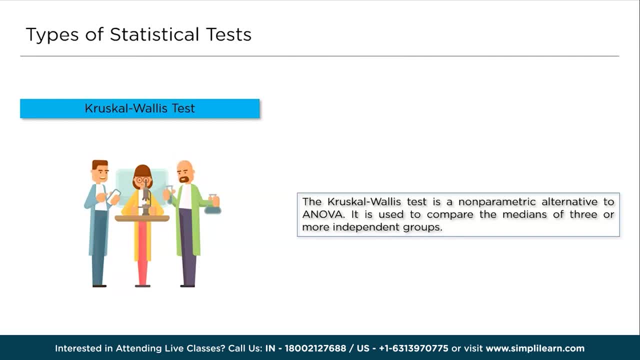 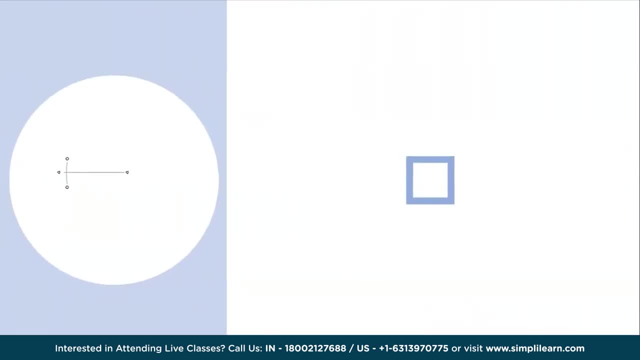 If the p-value is below a pre-determined significance level, it suggests that at least one group differs significantly from the others regarding the medians. Now the next one: Wilcoxon signed-rank test. This non-parametric test is used to compare paid samples and repeated measures. 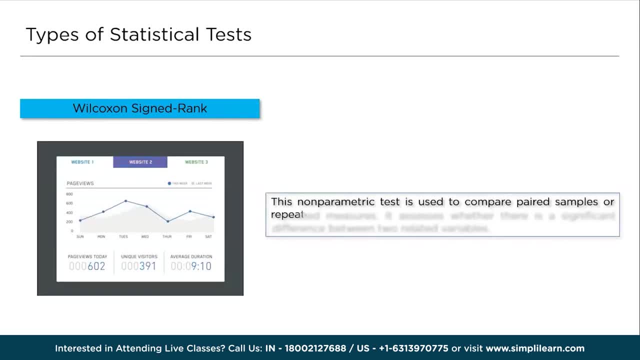 It assesses whether there is a significant difference between two related variables. The Wilcoxon signed-rank test is a non-parametric statistical test used to compare paired or matched samples. It is employed when the data do not meet the assumptions required for a parametric test. 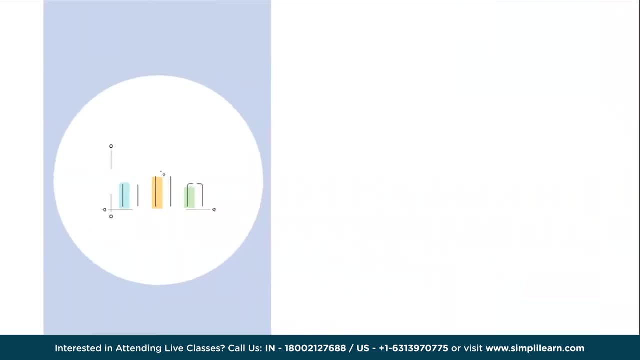 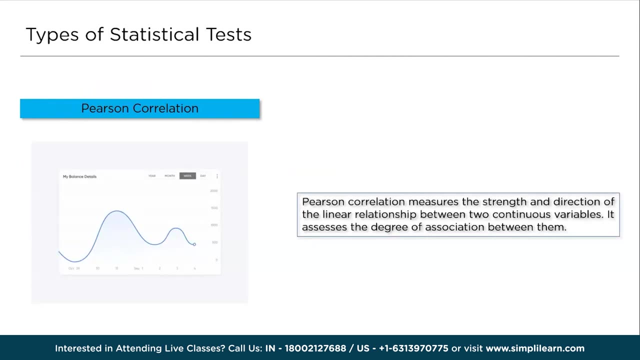 such as paired t-test. Moving ahead, we have Pearson correlation. Pearson correlation measures the strength and direction of linear relationship between two continuous variables. It assesses the degree of association between them. Pearson correlation is also known as Pearson's correlation coefficient. It is a statistical measure that quantifies the strength and direction of the linear relationship. 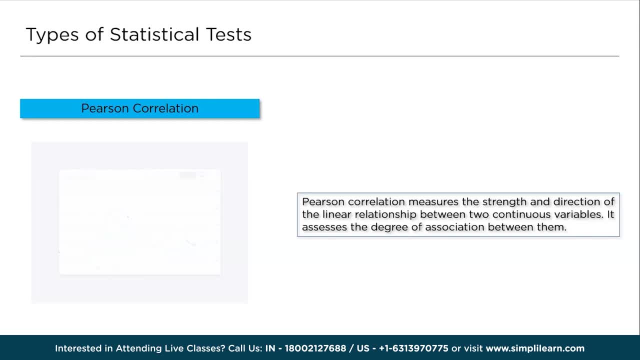 between two continuous variables. It ranges from minus 1 to plus 1, where minus 1 represents a perfect negative correlation and plus 1 represents a perfect positive correlation and zero indicates no correlation. Now, moving ahead, Let's move to the sixth part. 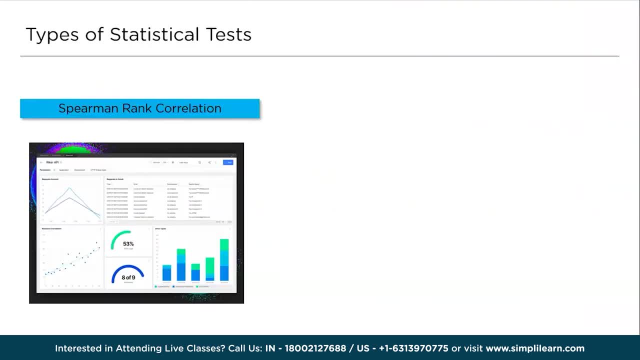 In the next position we have the Spearman Rank Correlation. The Spearman's Rank Correlation is a non-parametric measure of correlation that assesses the monotonic relationship between two variables. It is suitable for variables that may not have a linear association. 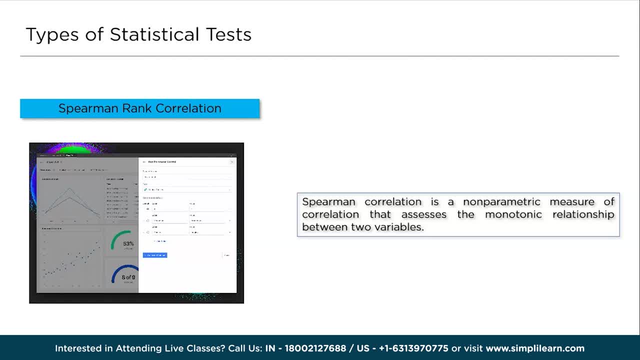 Spearman Rank Correlation is a non-parametric measure of correlation that assesses the monotonic relationship between two variables. It is used when the variables are measured on an ordinal or non-linear scale. This Spearman correlation coefficient ranges from minus 1 to plus 1, with minus 1 indicating 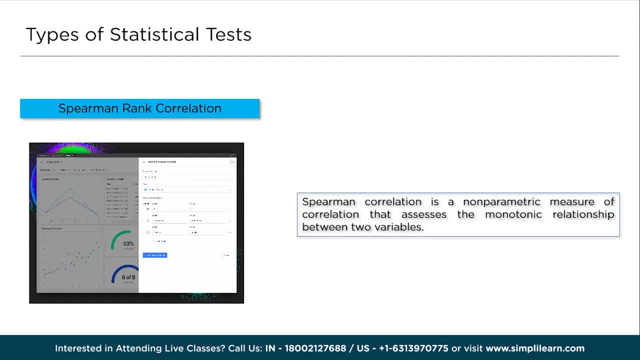 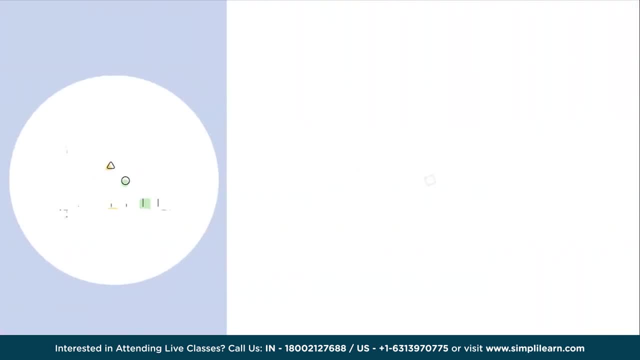 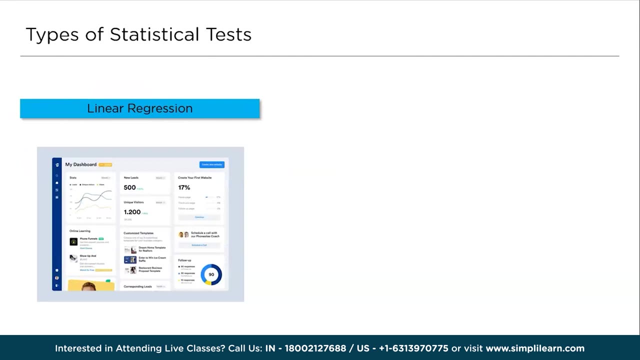 a perfect negative, monotonic relationship, and plus 1 indicating a perfect positive, monotonic relationship and 0 suggesting no monotonic relationship. Next, on the 7th position, we have Linear Regression. Linear Regression is used to model the relationship between a dependent variable and one or more. 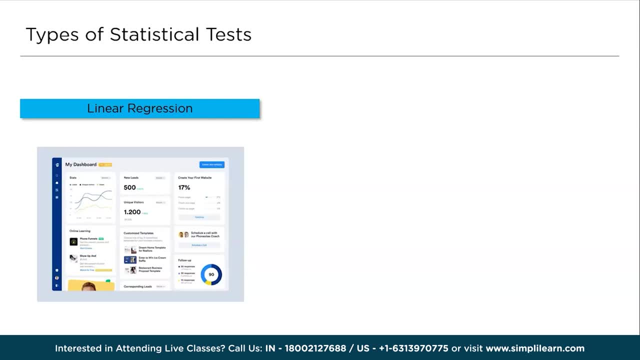 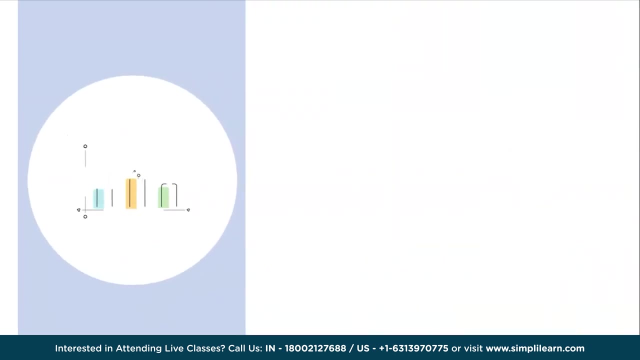 independent variables. It helps in understanding the impact of independent variables on a dependent variable. It assumes a linear relationship width to find the best fitting line that minimizes the sum of squared differences between the observed and predicted values. Moving ahead, we have Logistic Regression. 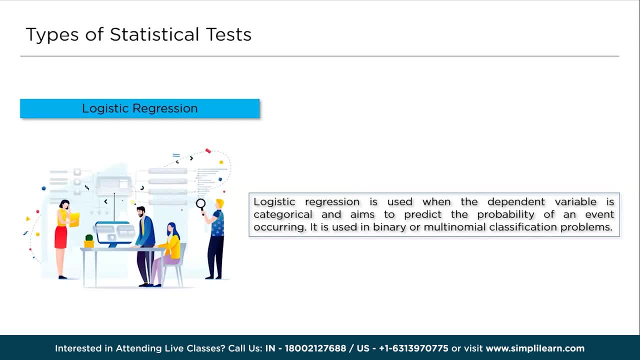 Logistic Regression is a statistical model that predicts binary or categorical outcomes based on one or more independent variables. It estimates the probability of an event occurring by force. It estimates the probability of an event occurring by force. It estimates the probability of an event occurring by force. 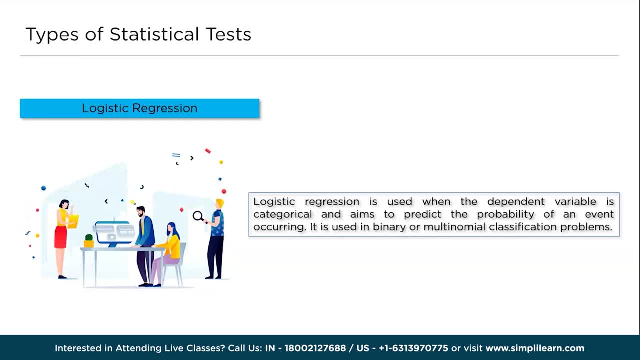 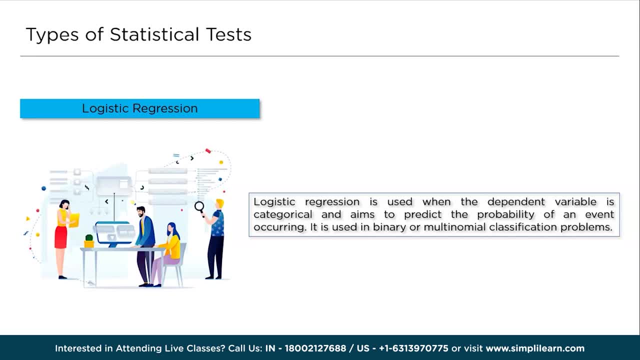 By fitting a logistic function to the data. Unlike Linear Regression, LG regression uses a linear combination of predictors into a probability. It calculates the odds ratio to measure the impact of each independent variable on the outcome. Moving ahead, we have Chi-square test. 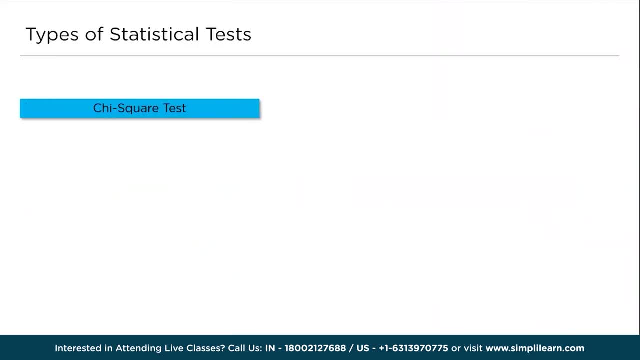 The Chi-square test is a statistical test used to determine if there is a significant association between categorical variables. It compares the observed frequencies of categorical data and the expected frequencies under the assumption of independence. The test calculates a chi-square statistic and generates a p-value. and if the p-value 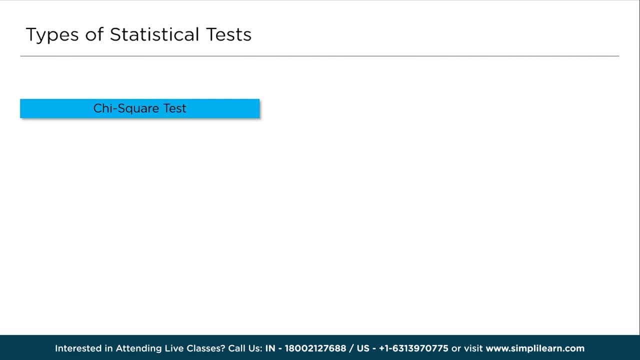 is below the chosen significance level, it suggests that there is a significant association between the variables. The chi-square test is commonly used to research areas such as social sciences, market research and genetics. to analyze data for goodness, to examine the independence between two or more variables. 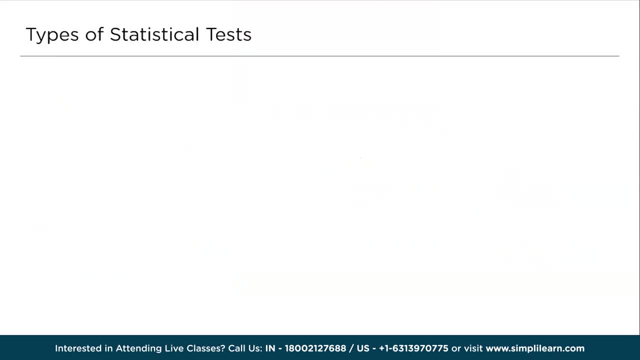 Next, the tenth one on the list, is Correlational tests. Correlational tests are statistical tests used to measure the strength and direction of the relation between two continuous variables. The most common correlational test is the Pearson's correlation coefficient, which assesses linear relationships. 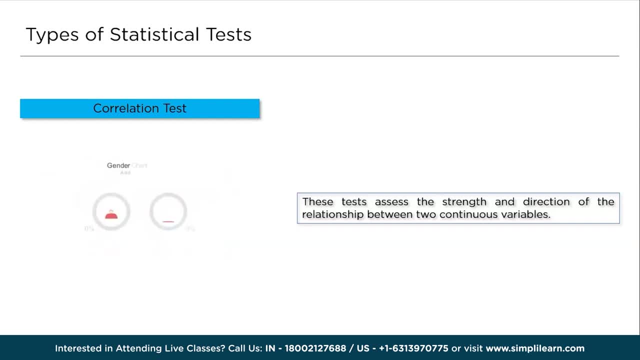 It ranges from minus one to plus one, where minus one indicates a perfect negative correlation and plus one indicates a perfect positive correlation and zero indicates no correlation. Other correlational tests include Spearman's rank correlation coefficient for assessing monotonic relationships and Kendall's rank correlation coefficient for measuring the 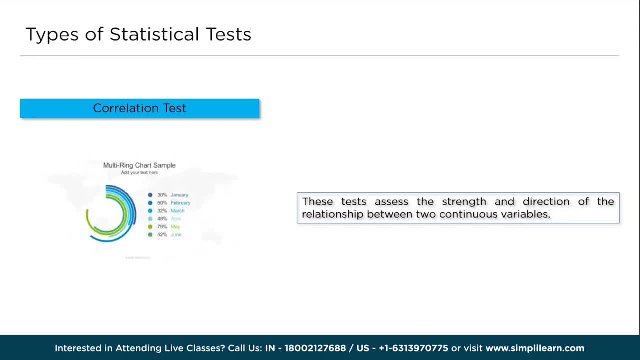 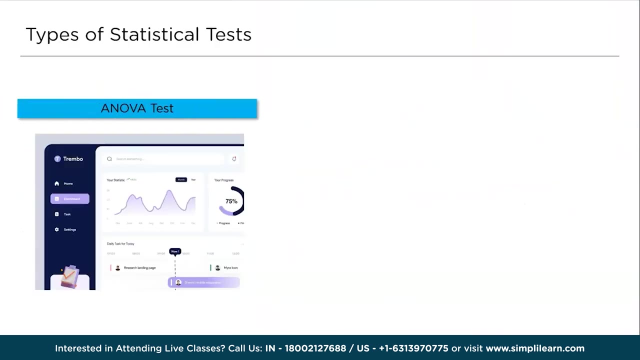 strength of association between the variables. Correlation tests help identify the degree and nature of the relationship between variables, aiding in understanding patterns and making informed decisions. Moving ahead to the eleventh position, we have ANOVA test. ANOVA, or Analysis of Variance, is a series of three analysis tests. 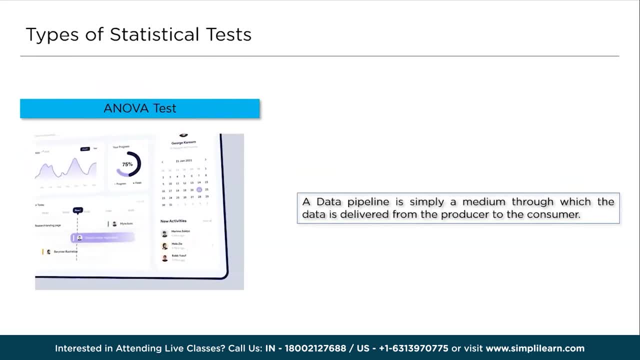 ANOVA, or Analysis of Variance, is a series of three analysis tests. ANOVA, or Analysis of Variance, is a series of three analysis tests. We try different things throughout the analysis process. w eth-STAT, Anova assesses the variation within and between groups, mae, calculating the f-static and generating 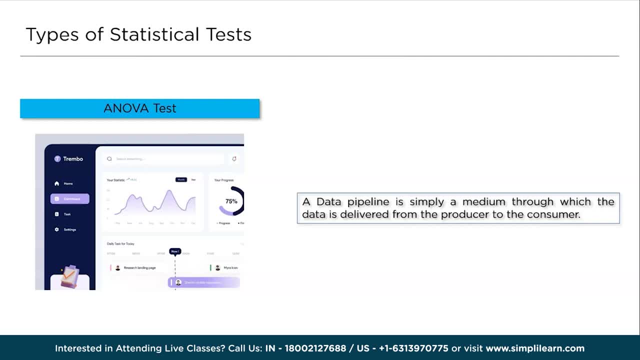 a p-value. If the p-value is below the chosen significance level, it suggests that at least one group's mean differs significantly from others data with multiple groups. It helps uncover differences and understand the impact of different treatments or factors on the response variable. Next we 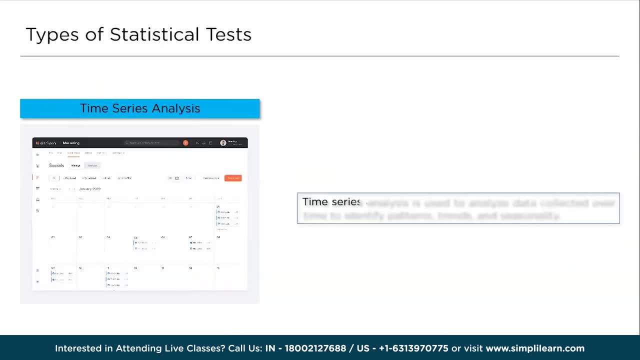 have time series analysis. Time series analysis is a statistical technique used to analyze and model data that is collected over time and at regular events. It focuses on understanding patterns, trends and dependencies within the time series data. The analysis involves exploring the temporal structure, identifying seasonality, detecting trends and examining 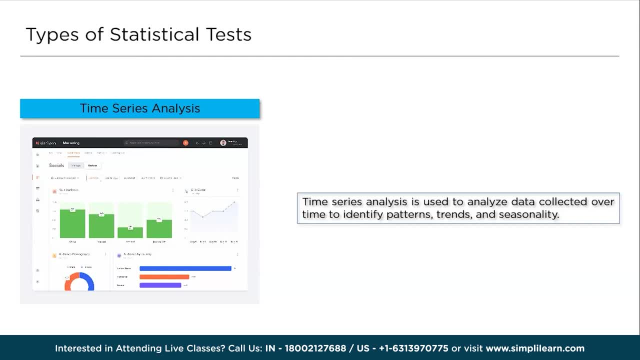 autocorrelation Time series models are IMA, that is, Auto Regressive. Integrated Moving Average and Exponential Smoothing are used to forecast future values based on historical patterns. Time series analysis is widely employed in various domains, including finance, economics, meteorology and stock market analysis, to 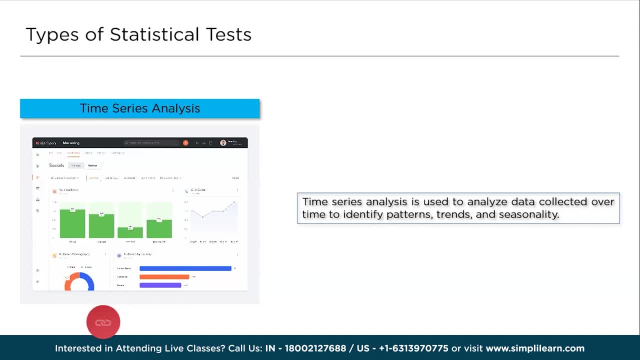 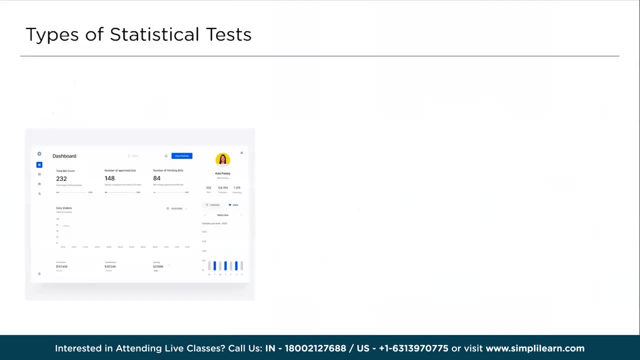 make predictions, identify anomalies and gain insights from time-dependent data. 13. Survival analysis. Survival analysis is a statistical method used to analyze time-to-time event data, where the focus is on the iteration until a specific event occurs. It is commonly applied in medical research, epidemiology and social 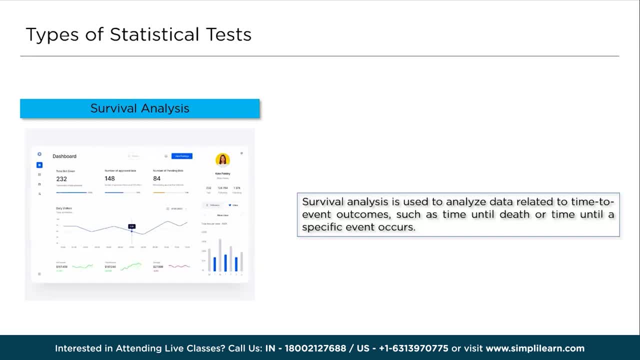 sciences to study survival times, such as time to death, relapse or failure. Survival analysis is used to estimate the survival probability over time. a log-ranked test to compare survival curves between groups and Cox Proportional Hazards Regression to assess the effect of co-varieties on survival. This analysis accounts for censoring, which 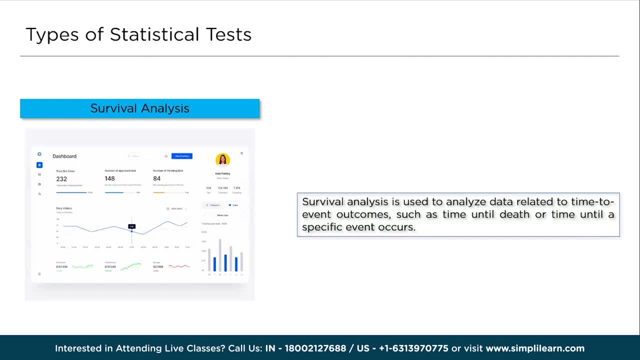 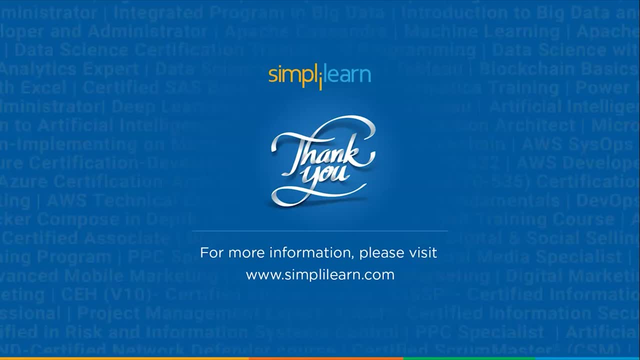 occurs when some individuals do not experience the event by the end of the study, providing valuable insights into the probability and timing of events of interest. And with that we have come to an end of this session on types of statistical tests. If you have any queries regarding any of the topics covered in this session, then please.